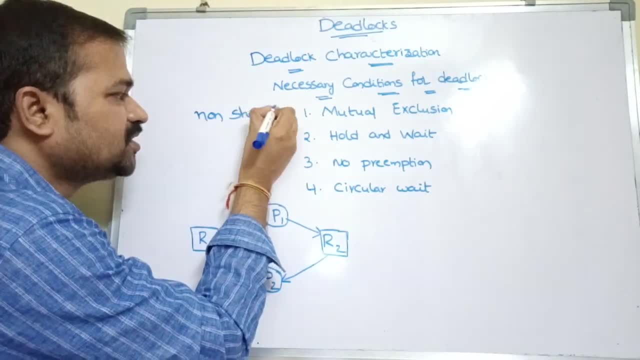 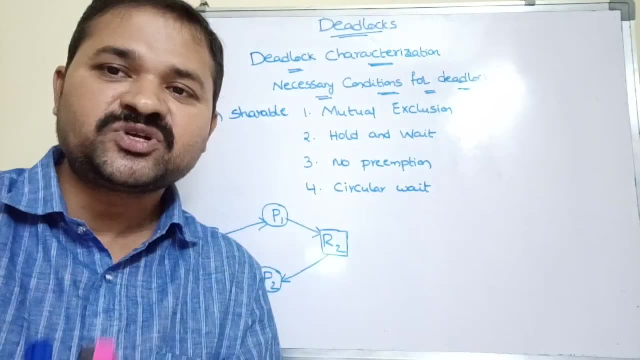 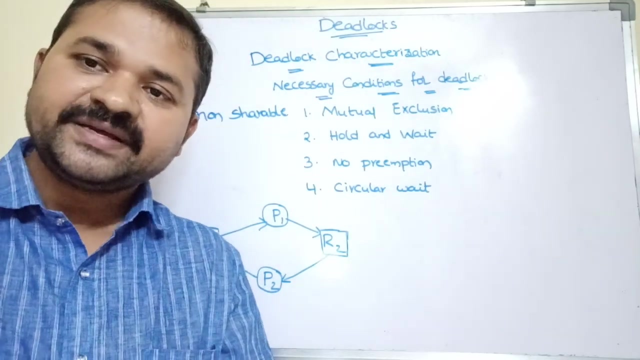 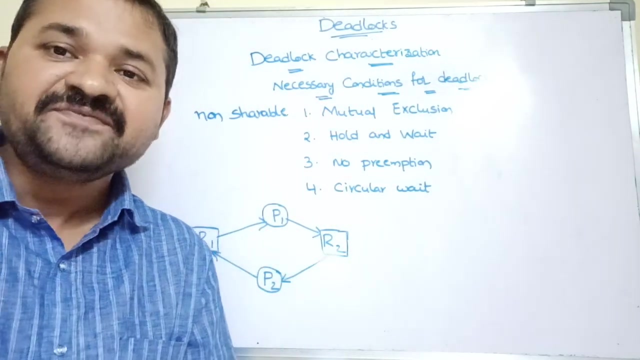 So by default it is not possible to share any resource among multiple processes. If we share a single resource simultaneously among multiple processes, then it will lead to wrong results. Assumes that we shared a printer between two processes simultaneously, then we will get the printing. 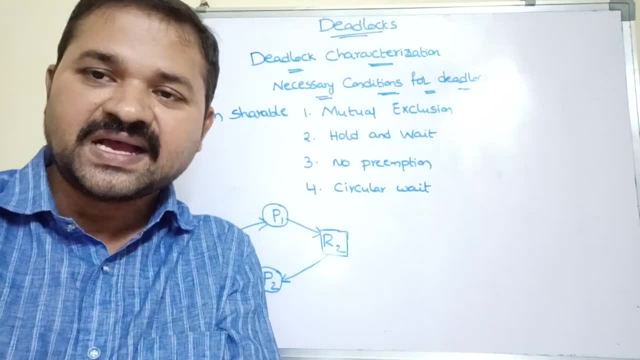 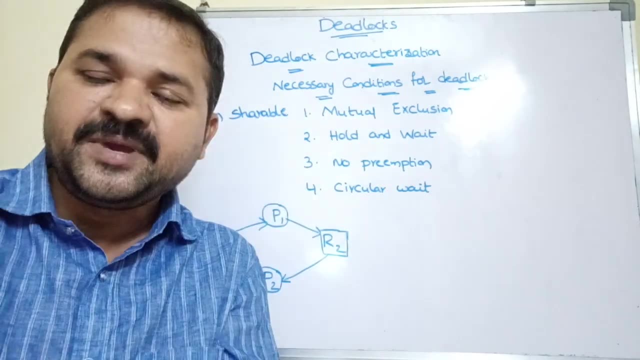 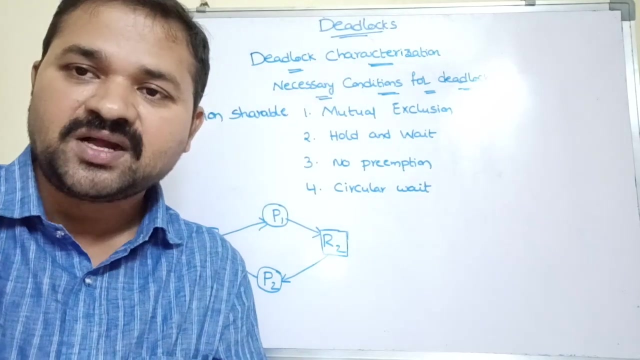 as the combination of those two processes. Here let the processes are P1 and P2. Let's say P1 and P2. And printer is shared among P1 and P2. Then printer produces both P1 process and P2 process combination as the output. So that means it is producing some wrong result. 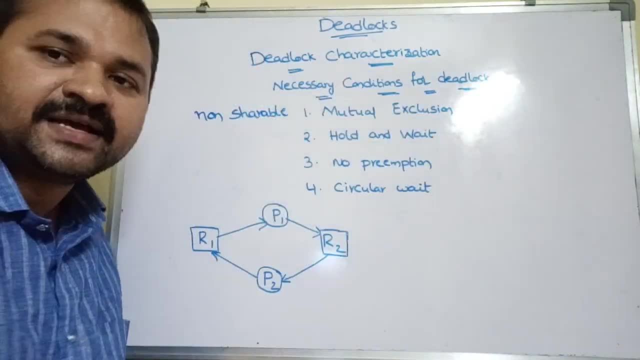 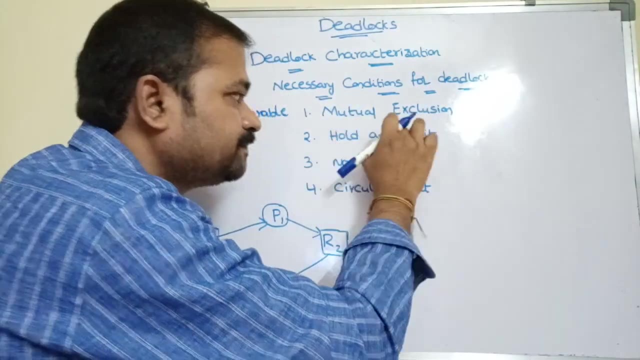 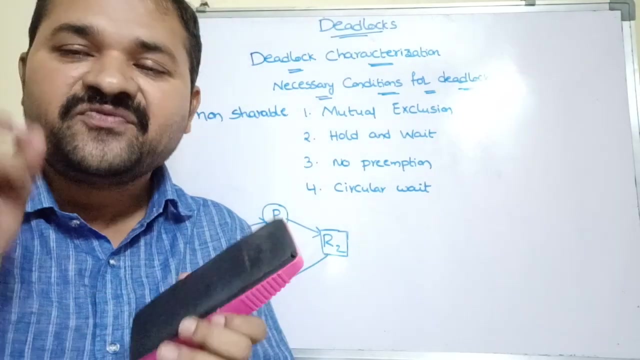 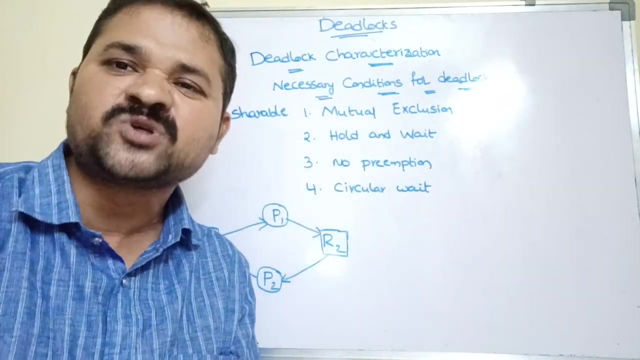 So here, if mutual exclusion occurs, then there is a possibility that deadlock may occur. So if we eliminate mutual exclusion, then we can say that there is no deadlock in the system. Eliminating mutual exclusion means we have to share a resource simultaneously among multiple processes. But practically it is impossible to share a resource among. 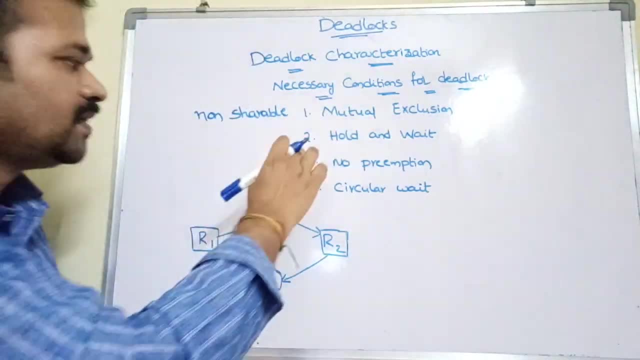 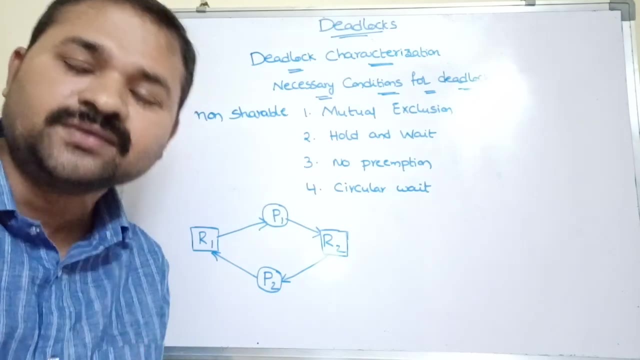 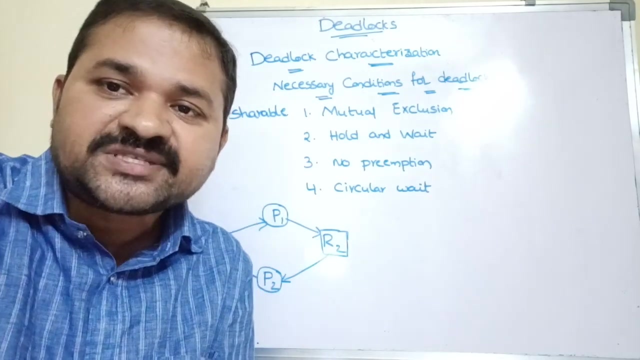 different processes simultaneously. And what is the second condition? Hold and wait. Hold and wait means a process is holding some resources and is waiting for additional resources, But those resources are acquired by some other process. If you take this example, P1 is: 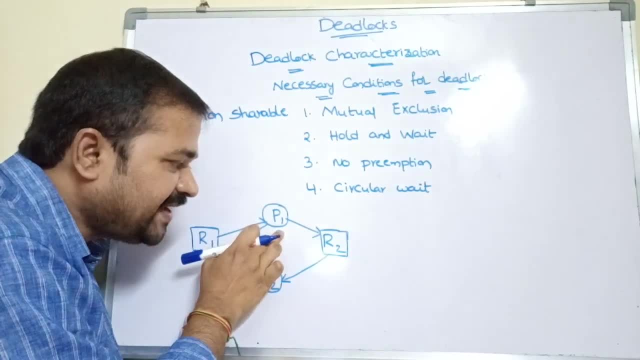 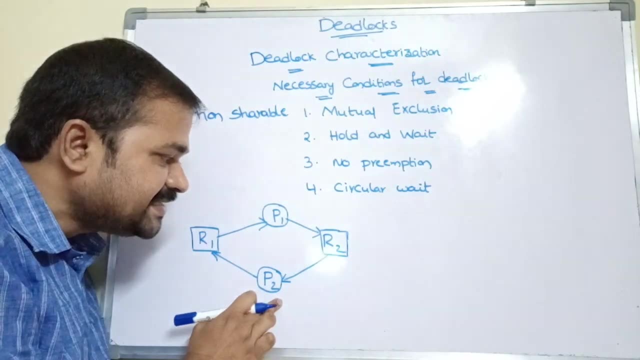 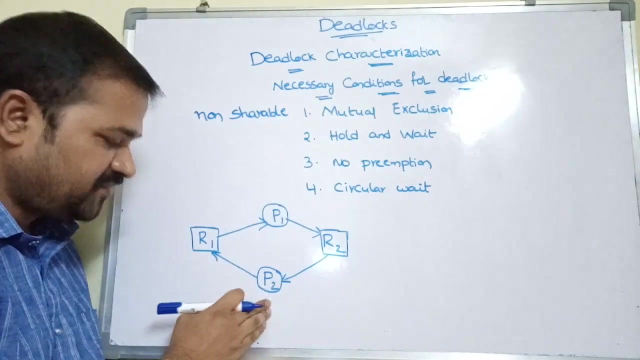 holding R1 and it is waiting for R2.. But R2 is acquired by P2.. P2 can release this R2 only after its completion. If you take about P2, if you consider about P2, P2 is holding R2. 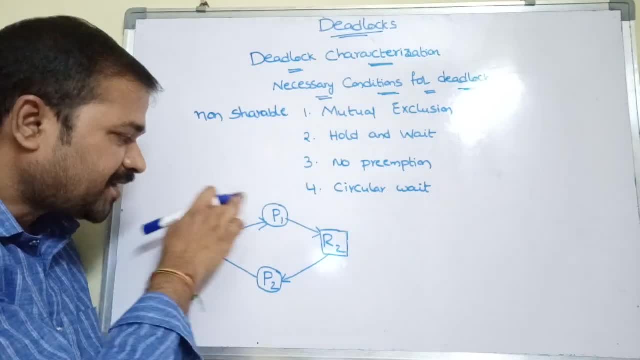 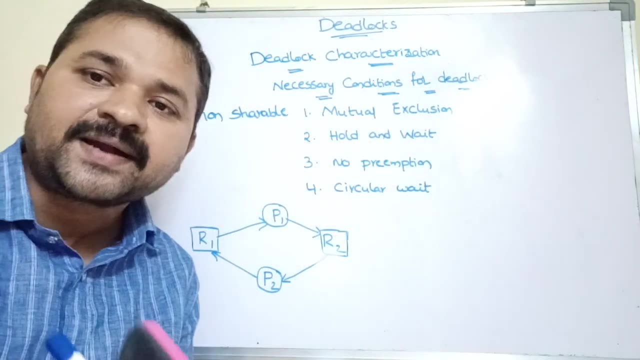 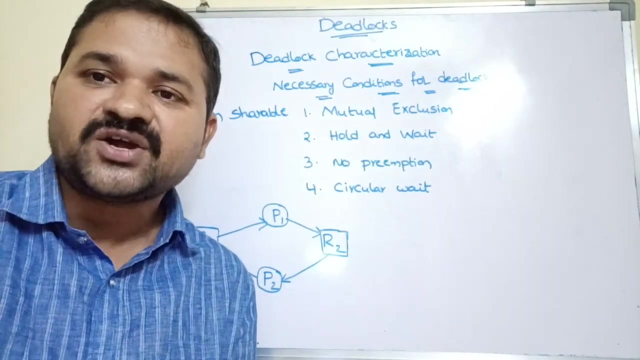 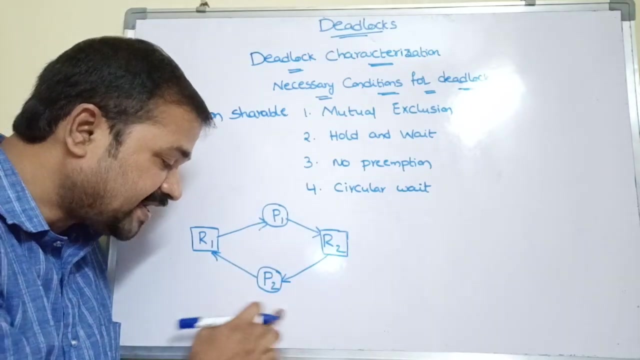 and is waiting for R1. But R1 is acquired by P1. So because of hold and wait, deadlock may occur in the system. If there is no hold and wait, then we can say that there is no deadlock in the system. Here P1 is holding R1 and it is waiting for R2.. If you consider, 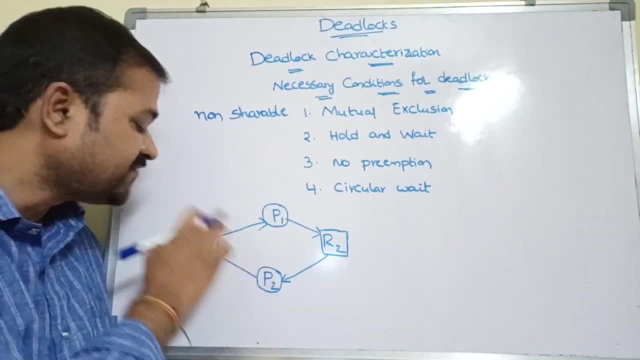 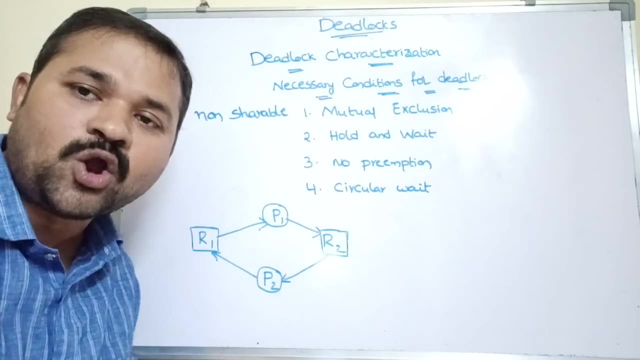 P2, P2 is holding R2 and is waiting for R1. So here we have hold and wait condition. So because of this hold and wait condition, deadlock may occur in the system. If we eliminate hold and wait, then there is no deadlock. 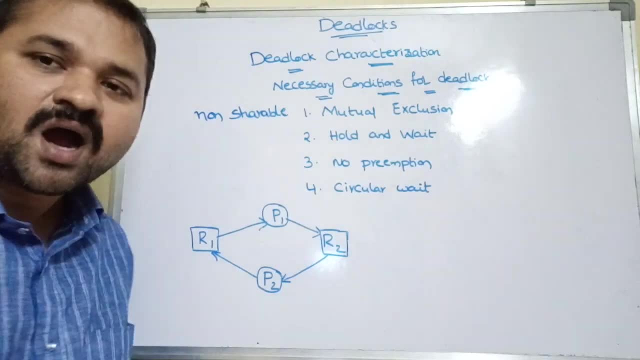 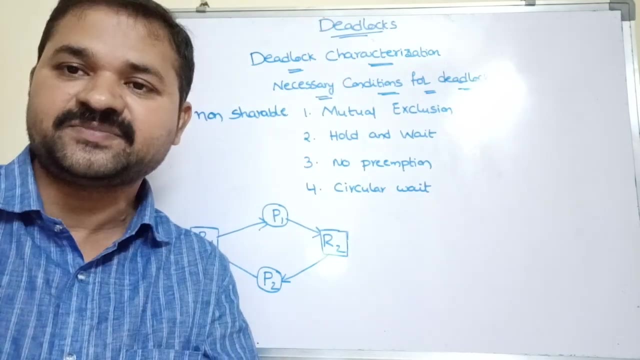 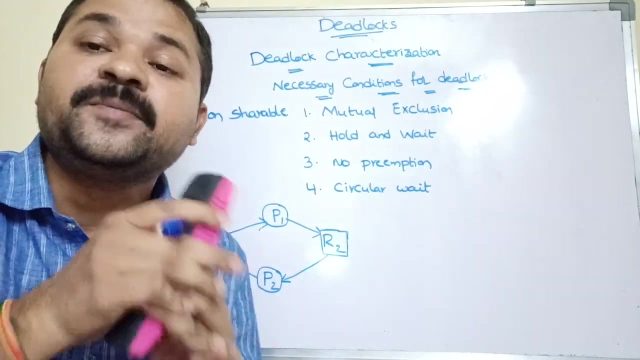 Now let us see about the third condition, that is, no preemption. Already we know about primitive CPU scheduling algorithms and non-primitive CPU scheduling algorithms. So primitive CPU scheduling algorithm means during the execution CPU can primp a process, So the CPU can primp. 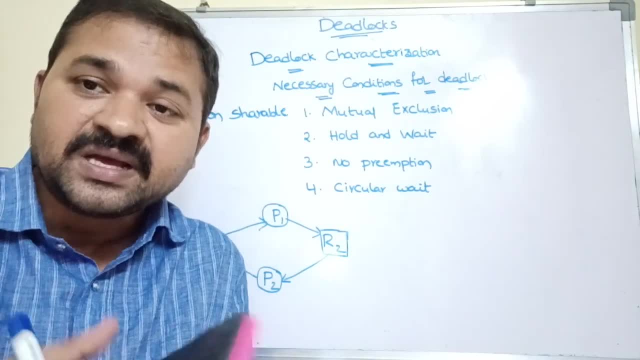 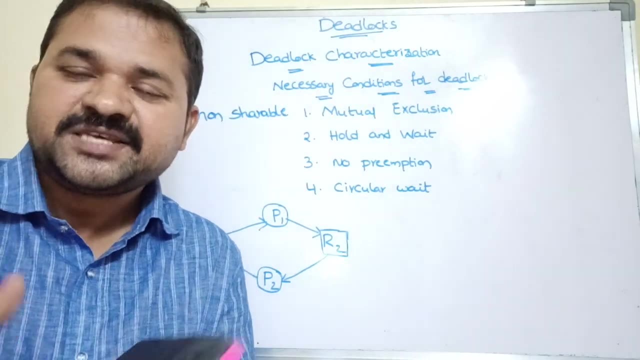 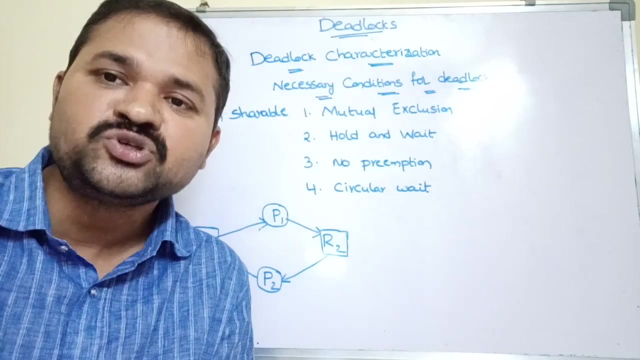 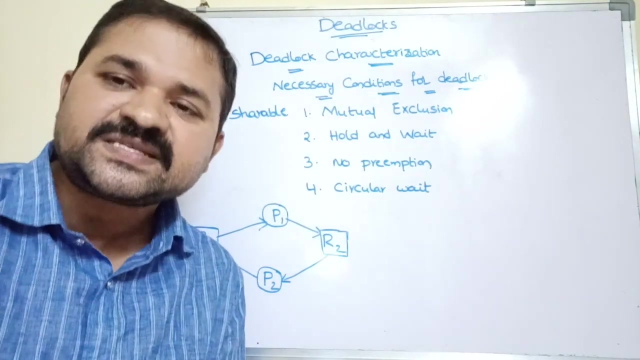 a process. That means CPU can stop the execution of a process. If you take non-primitive CPU scheduling algorithm, then CPU cannot stop execution of a process. So that is about primitive and non-primitive CPU scheduling algorithm, Whereas here we have no preemption. So no preemption means a process cannot release. 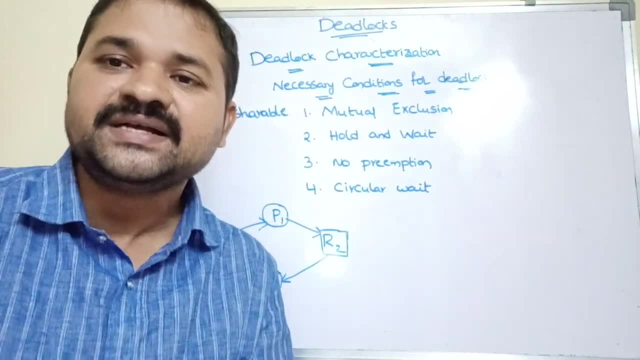 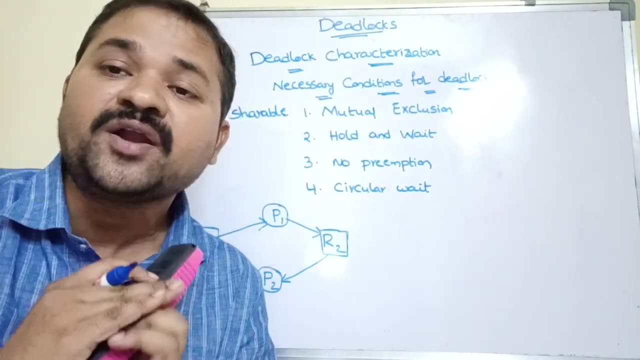 a resource until and unless a process is executed. So no preemption means a process cannot release a resource until and unless a process is executed. So no preemption means a process cannot release a resource until and unless a process is executed. It has completed its execution. So during the execution a process cannot release the. 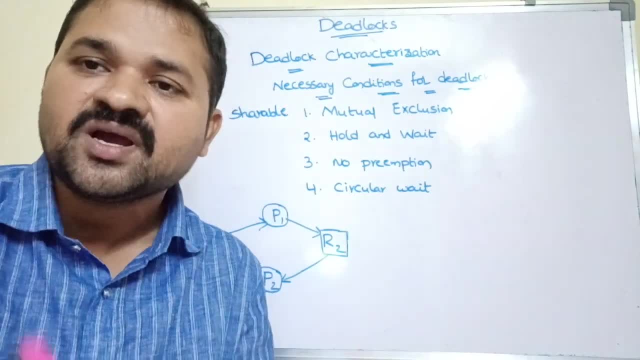 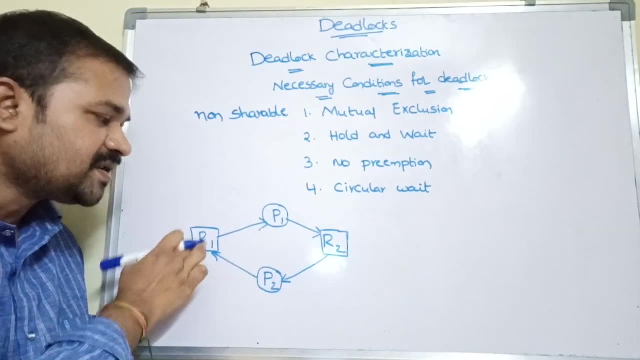 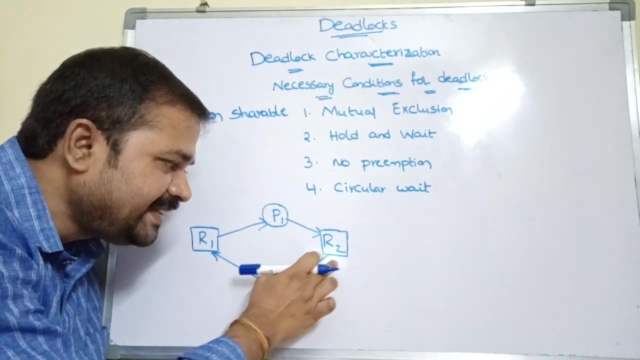 resource. A process can release the resource only after completing its execution. If you take this example, P1 releases R1 only after completing P1 execution. If we consider here about P2, P2 can release R2 only after completing P2 execution. 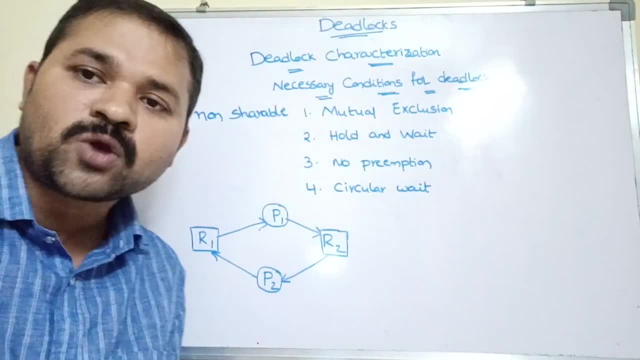 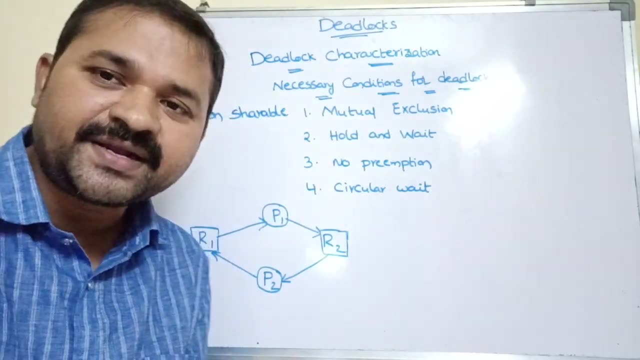 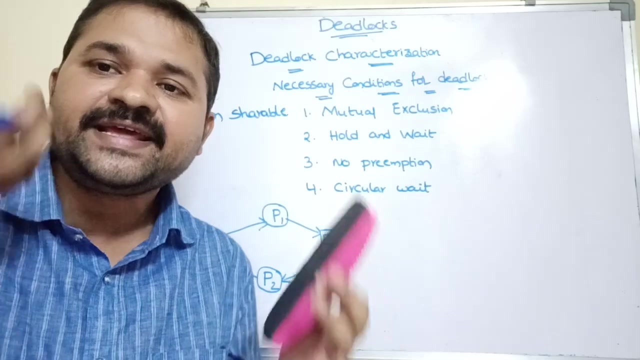 So because of no preemption, deadlock may occur in the system If we eliminate no preemption. eliminating no preemption means what? If the process releases the resource during the program execution, then we can say that there is no deadlock in our system. Now let's see about. 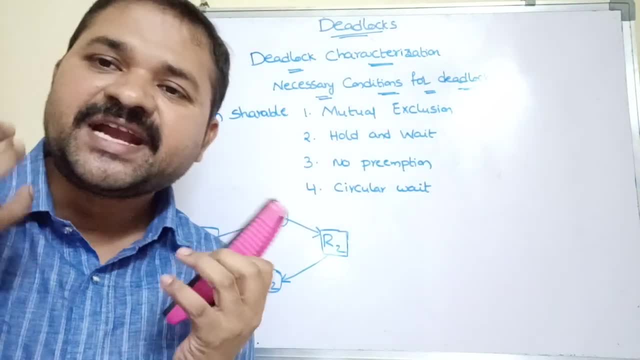 the last condition, that is, circular wait. A set of processes are said to be in the deadlock state. If one process releases R1, R2,, R3,, R4,, R5,, R6,, R7,, R8,, R9,, R10,, R11,, R12,, R13,, R13, R14,,